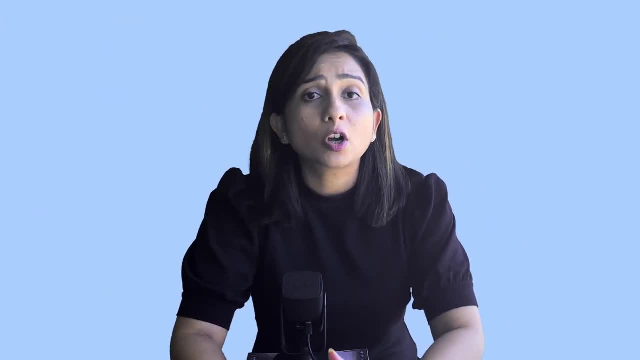 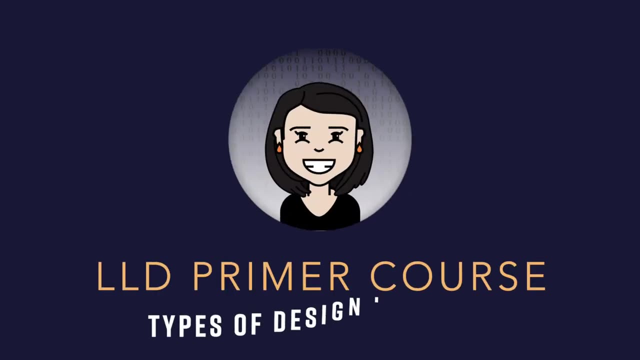 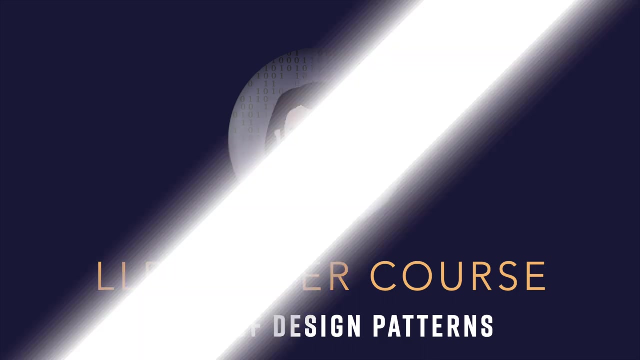 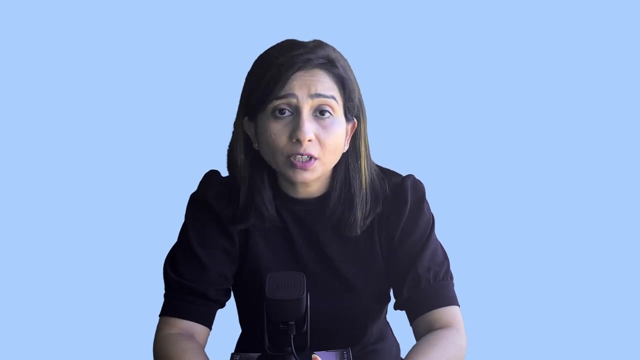 make you comfortable enough to work with it. Now let's talk about the organization and different types of design patterns, Since design patterns solve the problem of how you're going to organize your classes and objects and their behavior and their communication between each other. we can actually break design patterns in terms of those categories. 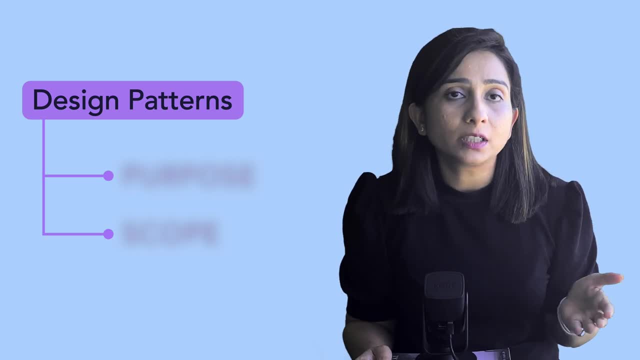 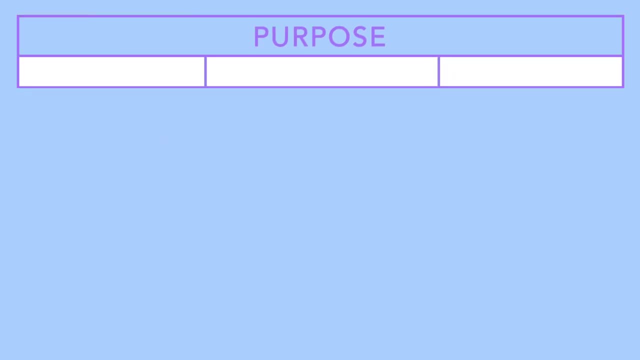 So the first criteria on which we divide different design patterns is the purpose. What is the purpose any design pattern solves? Now there can be three purposes that any design pattern would be solving. First is creational purpose. Whenever you want to create classes or objects, or instantiate objects of classes there, 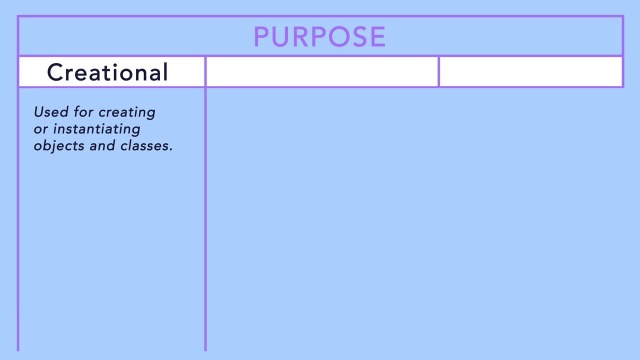 comes the creational design patterns, and different design patterns which come under the creational category are described here. Next category is the structural category, and that's why those are called structural design patterns. When we talk about structure, that means how we are going to structure. 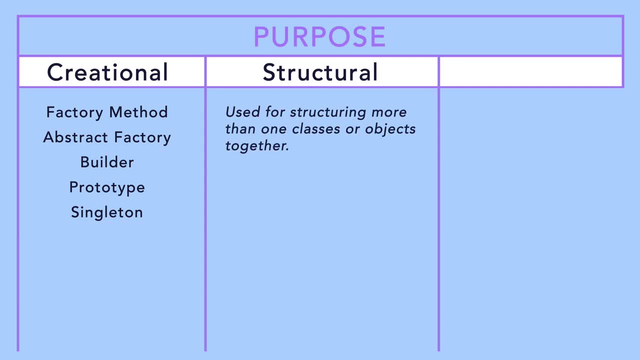 more than one classes and objects along with each other. It includes different, different ways in which we can use inheritance. it will also touch upon the interface segregation principle that we have discussed. how do we design our interfaces? So all those structuring that we do around objects and classes, those 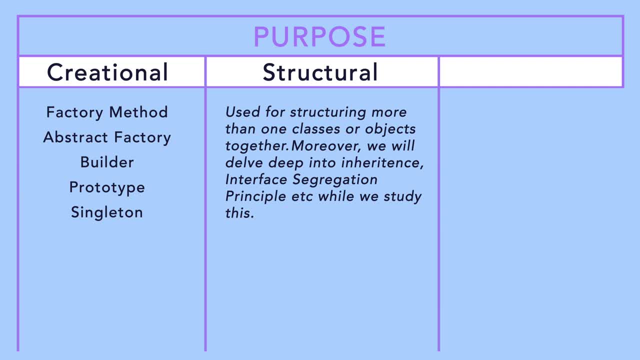 patterns. solving such kind of structural problems fall under the structural patterns, and the patterns which follow under structural category are here, and the final criteria is the behavior. once we are done instantiating the objects and classes and once we are done structuring them in relation to each other, the last part that any object oriented code solves is actually those. 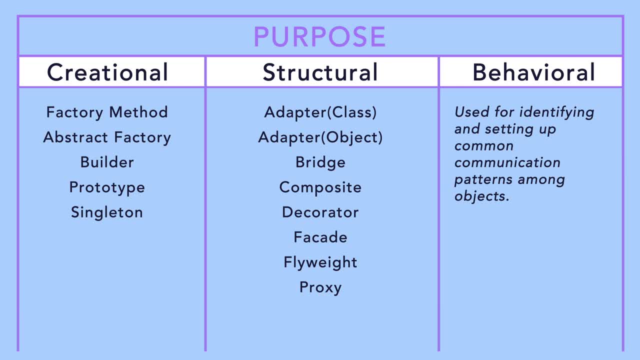 objects and classes communicate with each other. they pass messages to each other in order to fulfill a complex business use case, or in order to fulfill a use case like saving the data or fetching data, etc. that behavior is actually solved using the patterns which we categorize as behavioral patterns. 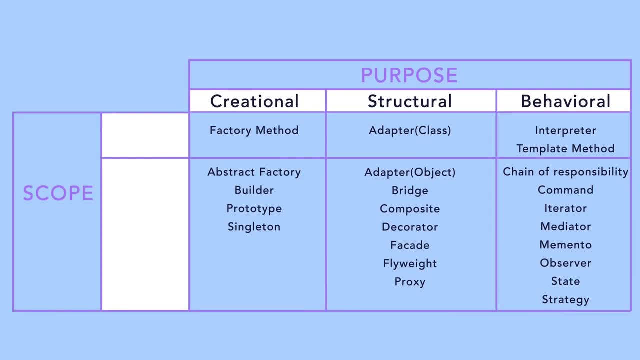 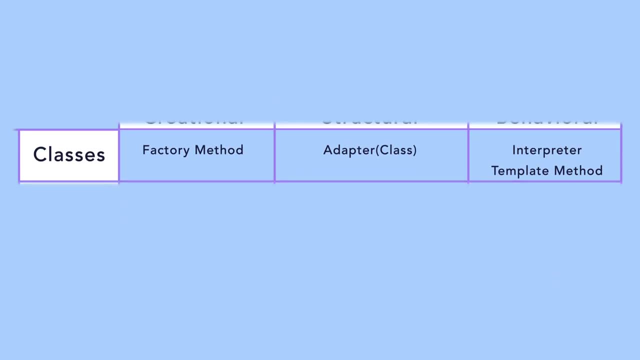 which you can see here. now there is also a way to categorize these patterns: on the basis of classes and objects. there are some patterns which will be applicable only on objects, and there are some patterns which will be applicable only on classes. actually, mostly all the patterns work on objects. there are only 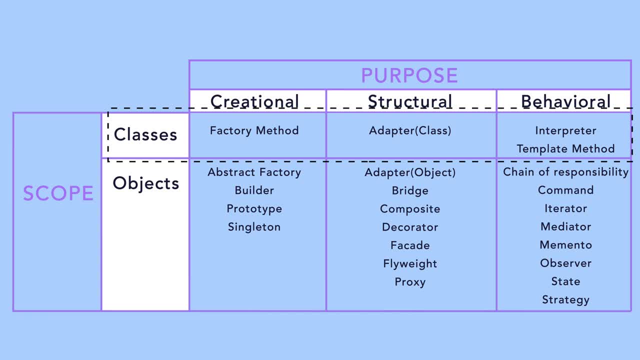 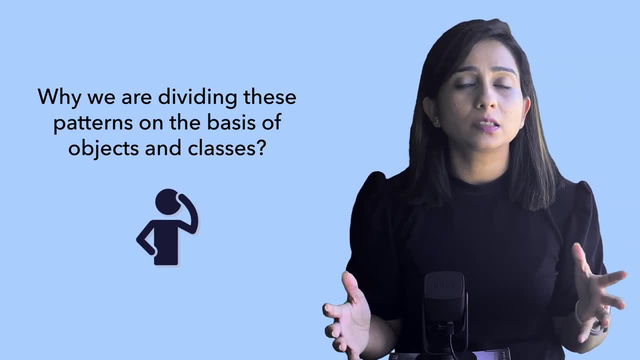 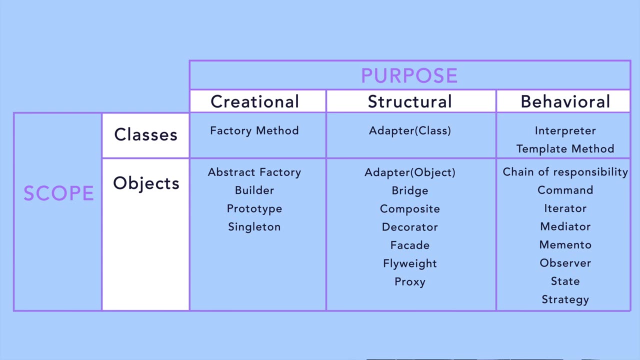 four or five patterns, as you can see here in the list, that are applied on classes rest. all the patterns are actually applied on the objects. now why we are dividing these patterns on the basis of objects and classes. here is why, if you look at the creation patterns which cater to class, that means those 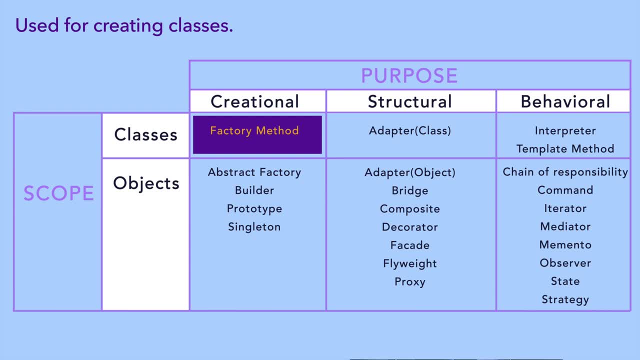 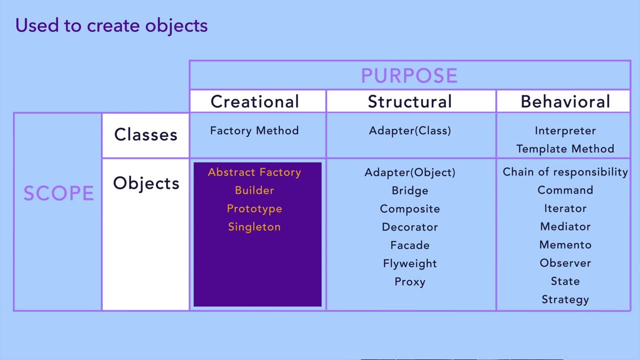 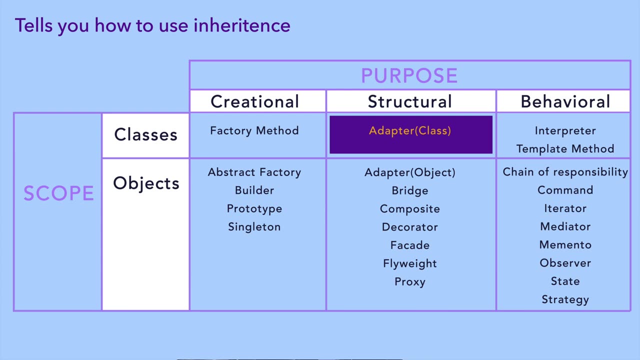 patterns are actually telling you how to create classes. if you talk about creation patterns categorized under objects, those patterns are actually telling you how to instantiate objects for different classes. similarly, the structural patterns that we have categorized under classes and objects- the structural class patterns- actually tell you how to use inheritance. 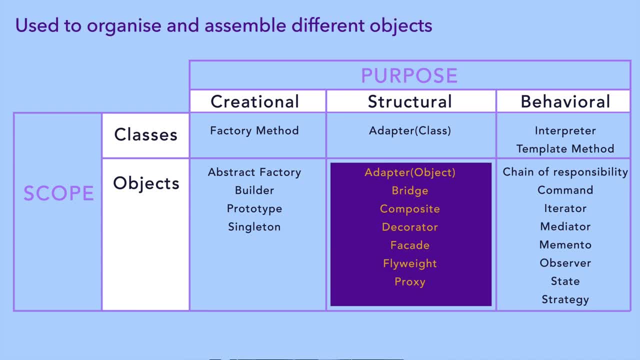 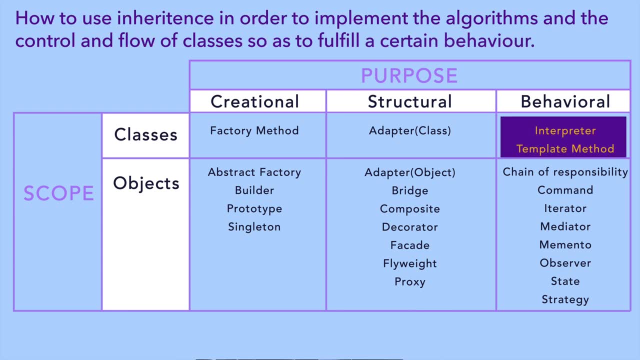 and the structural object pattern actually tried to tell you how to organize and assemble your objects. similarly, behavioral patterns- the behavioral class patterns- actually tell you how to use inheritance in order to implement the algorithms and the control and flow of classes so as to fulfill a certain behavior. and behavioral object patterns actually tell you how to. 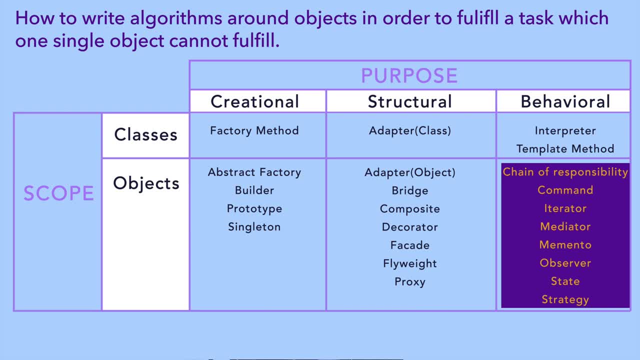 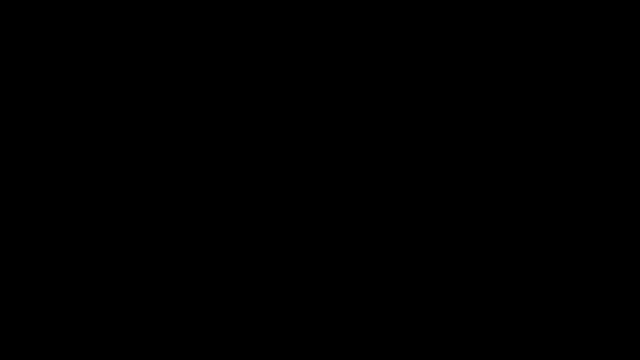 assemble and how to write algorithms around objects in order to fulfill the task which one single object cannot fulfill. so, basically, if there are multiple objects that are included to fulfill a certain behavior, the behavioral patterns pertaining to objects solve those kind of problems. the reason that we are discussing this organization of different patterns is 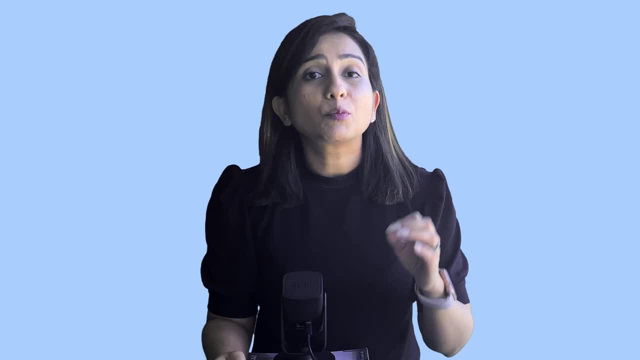 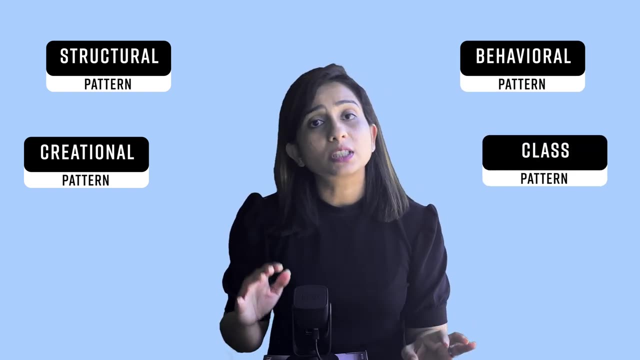 because now, when we are going to actually study a pattern, I am going to use terms like: this is a creational pattern, or this is a structural pattern, or this is a behavioral pattern, this is a class pattern or this is an object pattern. just if you understand this structure. 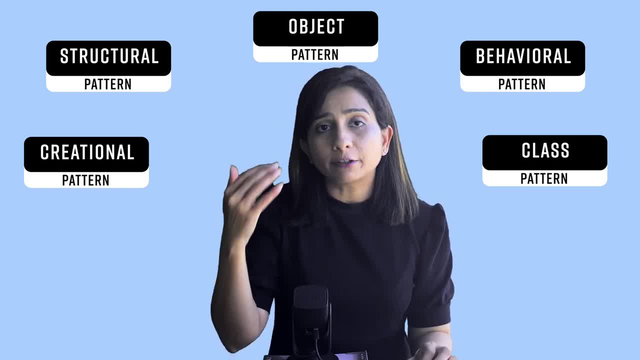 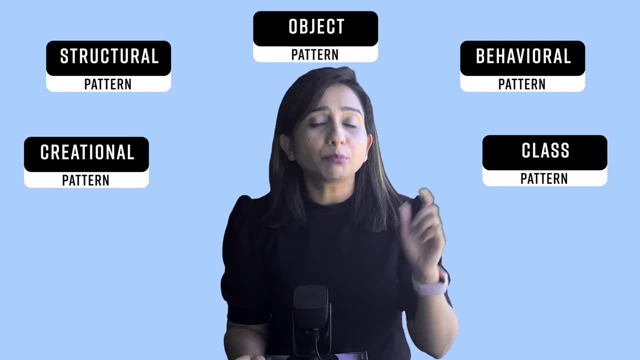 that we have discussed today, when we are going to address different patterns as a structural or creational patterns, or structural class patterns, you would be able to understand what exactly I mean by that and also you would be able to create a mental map of this categorization, so it would be easy for 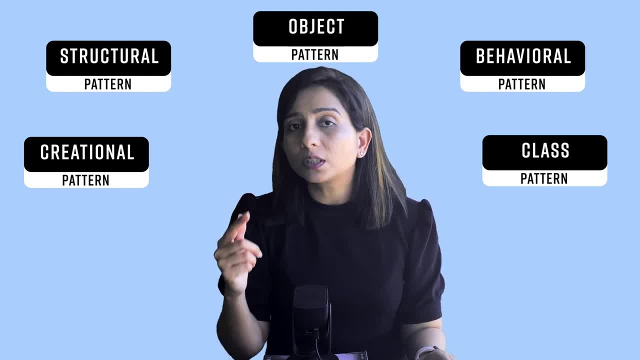 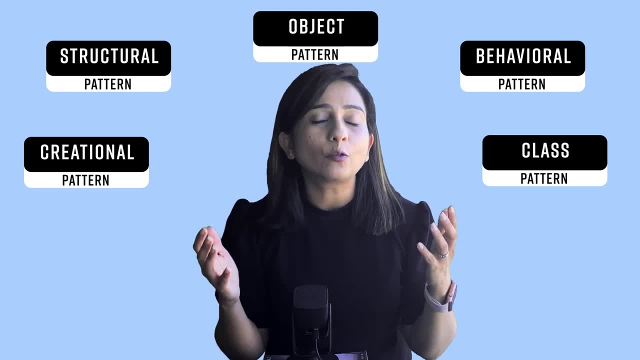 you to look at a pattern and understand exactly why is it important that you are, what kind of problem this pattern might be solving. it is not a memorizing technique, but it is just a technique to ease you into the process of learning design patterns. now to summarize, before we 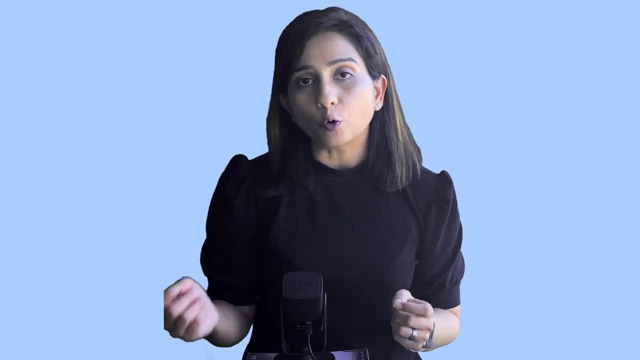 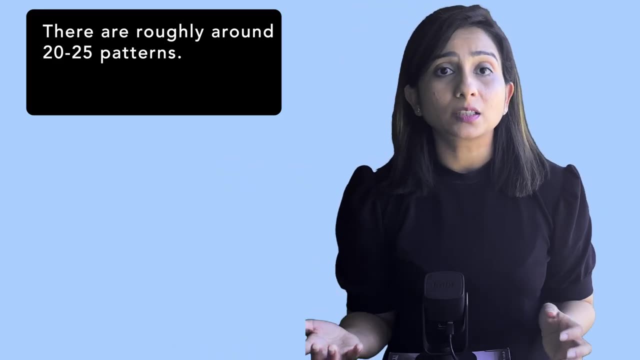 actually start picking each pattern and write code and understand code for each pattern. i want to highlight certain points. there are roughly around 20 to 25 patterns. there can be more patterns upcoming with new tech, with new technology and new languages. please try to understand that you. 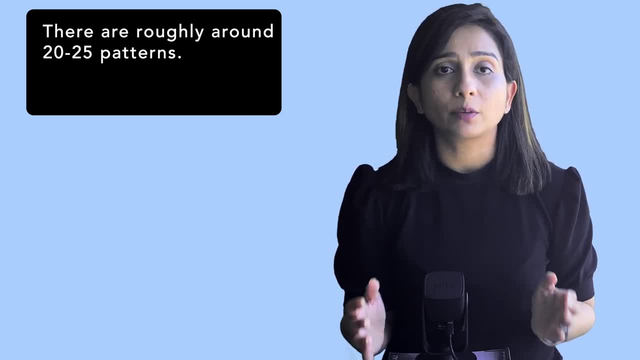 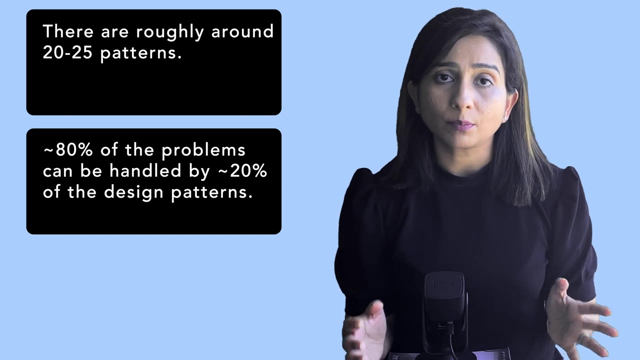 will not be able to memorize all 20-25 patterns by heart and also you are not going to use all 25 patterns in even a single year of coding. there are some patterns. if you think about the 80-20 rule, there are 20 percent of the patterns that you are going to use 80 percent of the time and remaining 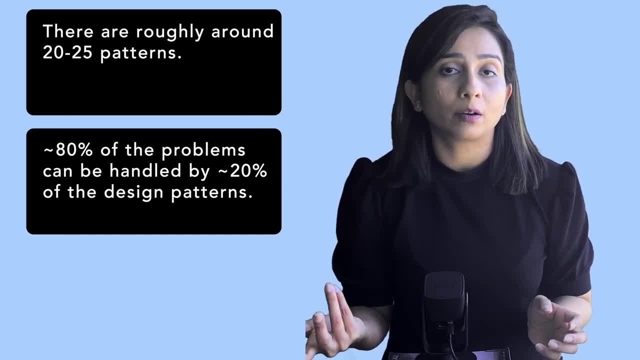 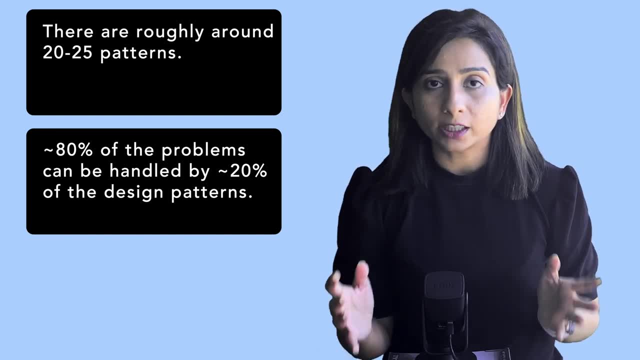 80 percent of the patterns you might be using may or may not be using in your journey. so what i would like to highlight is try to learn each pattern, try to understand each pattern, try to solve each pattern, and then you will be able to memorize all 20-25 patterns by heart, and also you. 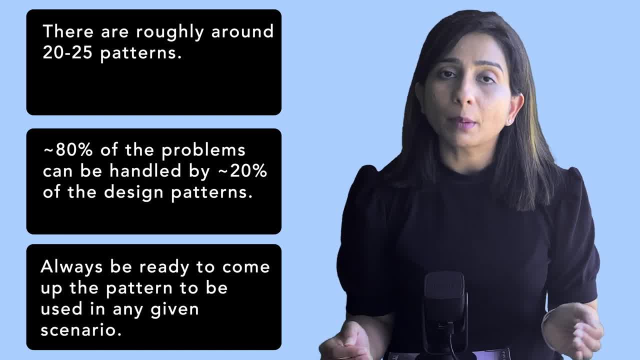 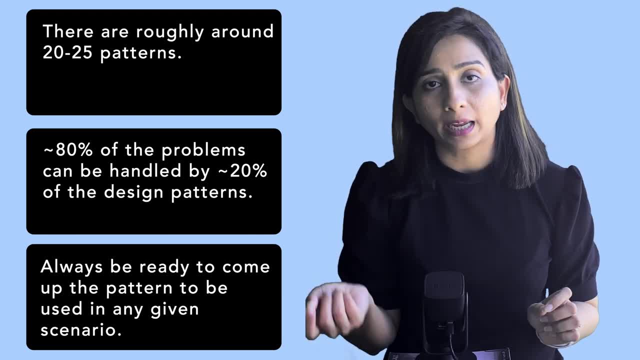 will be able to solve one or two problems with respect to every pattern and always remember, whenever you have to solve a problem, you should be able to go figure out which pattern would solve this problem and apply it. it is not necessary for you to know each and every pattern, it is only 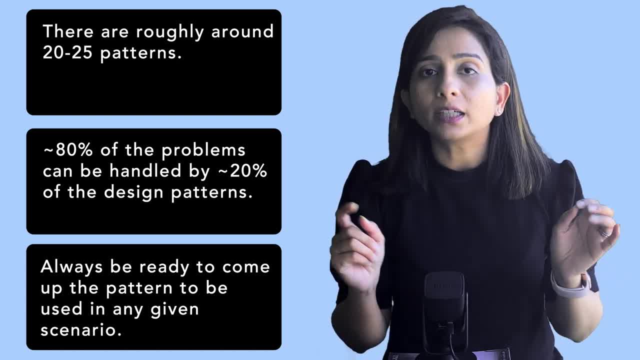 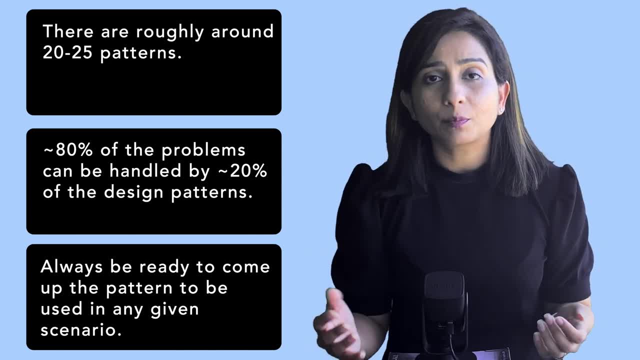 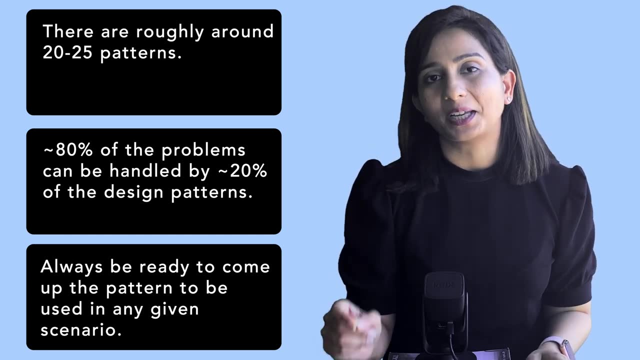 necessary for you to identify the problem, identify the pattern and map the problem and pattern. that is only thing which is required from any junior developer or senior developer or any developer. nobody expects you to remember all these things. the only expectation is you should be able to solve the problem in a right way. so keep this in mind while 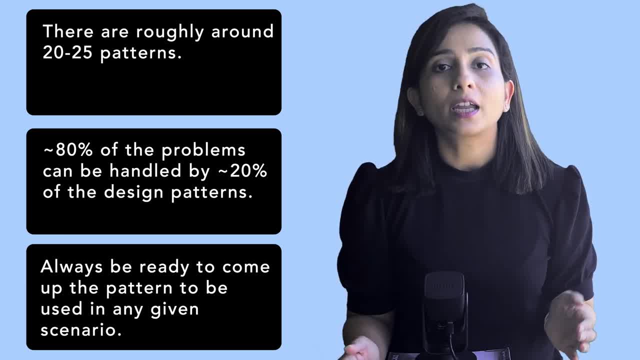 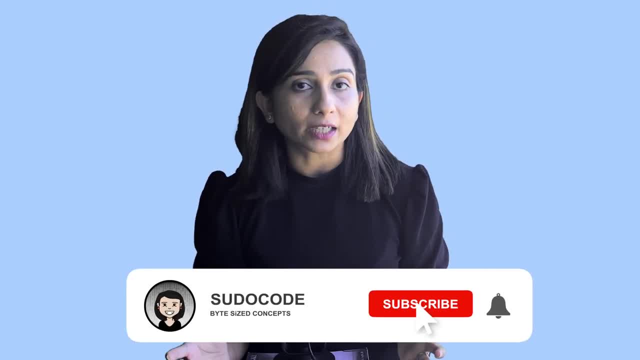 learning the patterns and i hope that you don't get overwhelmed by a series of so many patterns. so that was a brief introduction of different types of patterns and how you can learn patterns. from the next video onwards, we are going to dig deep into every pattern, using some examples and 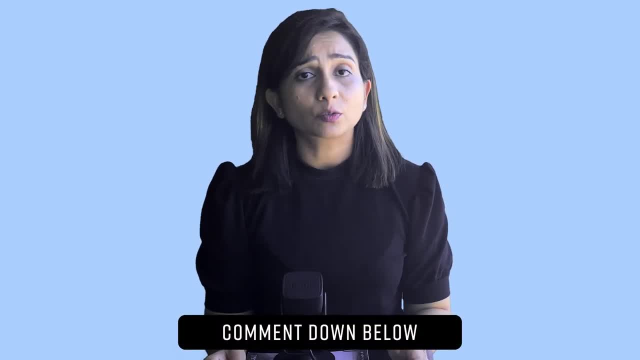 we will see what problems those patterns solve. if you have any doubt with respect to this video or if you have any other questions, please feel free to add them in comments. i have added different resources for this video and i will see you in the next video. bye, bye. 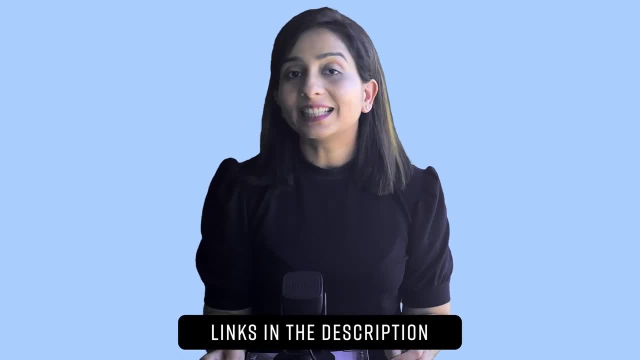 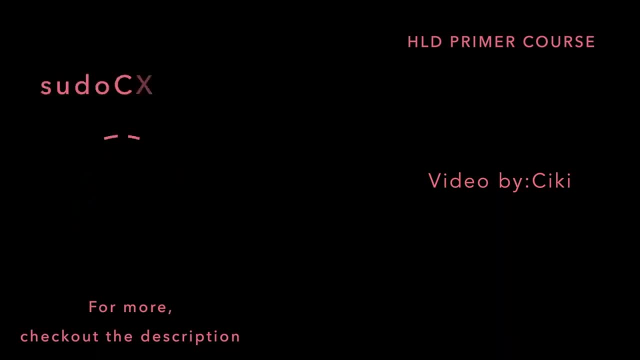 a video, please check the description. those are linked in the description. in the next video we will discuss factory patterns. till then, take care. see you in the next video.